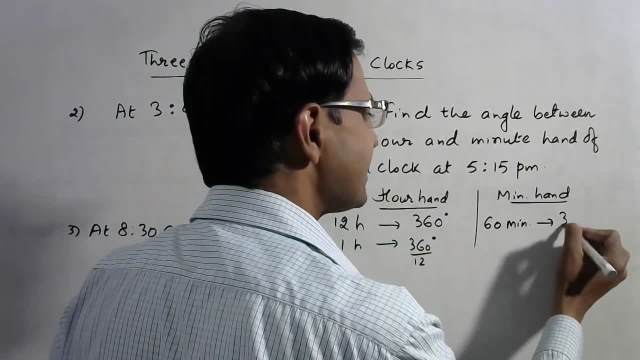 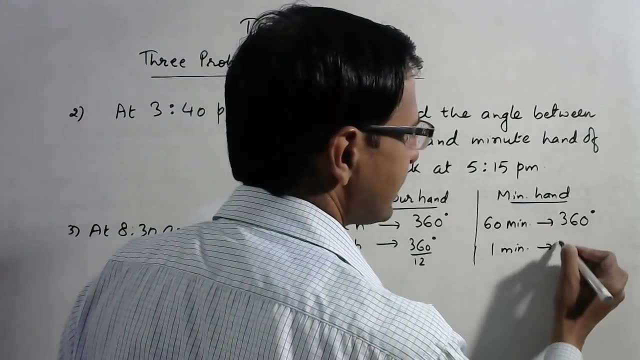 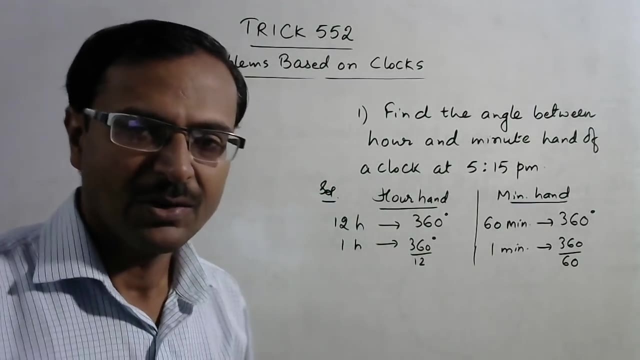 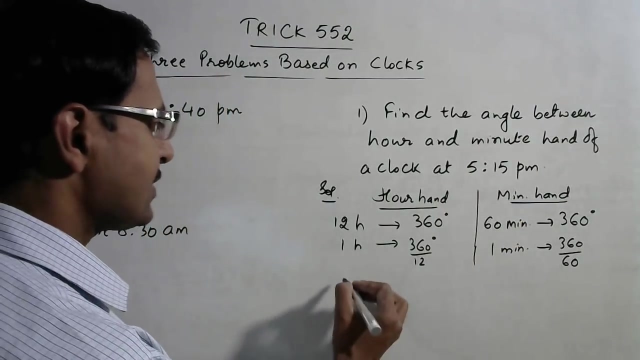 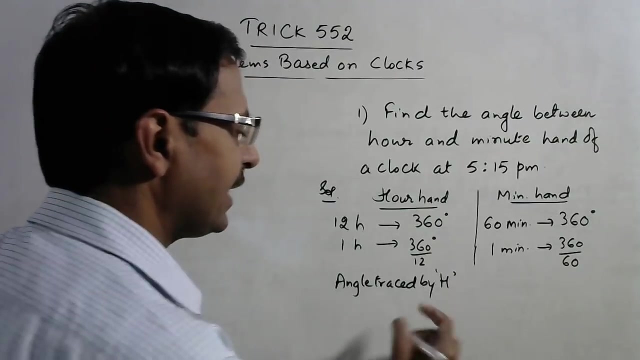 minutes, the angle traced is 360 degree. So in one minute the angle traced is 360 upon 60, that is, 60 degree. Now, this is the concept we need to understand when we solve such questions. Now, what happens when the time given is 5- 15 pm? Now see angle traced by hour hand. I am writing. 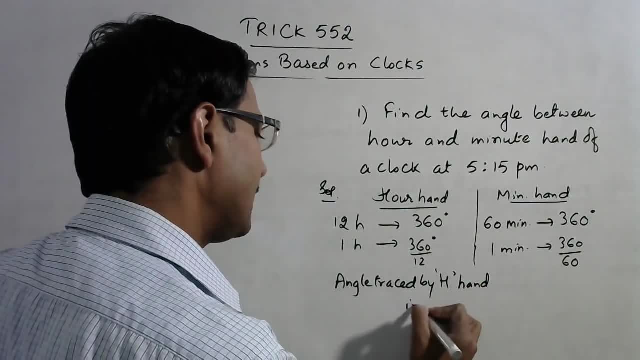 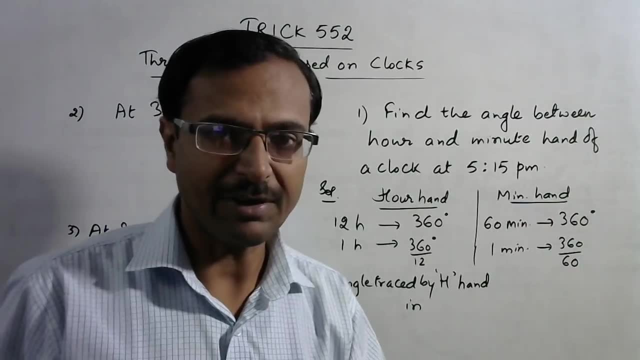 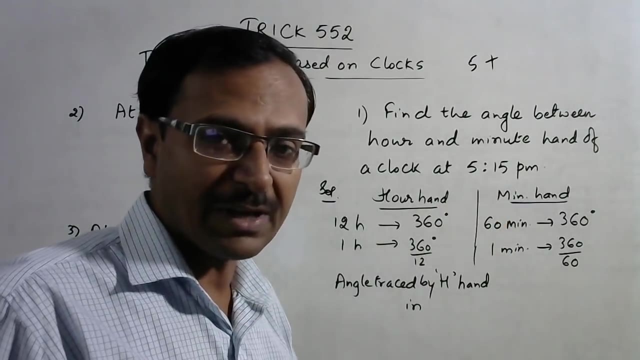 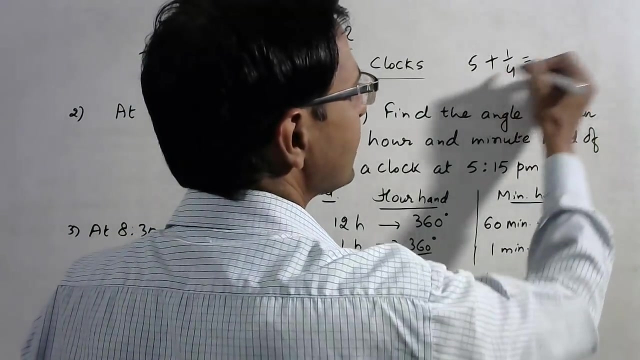 capital H hour. hand in now. how much time Now. 5, 1 by 5, 5, 15 pm. 5: 1, 5 pm. So 5 hours is cleared plus 15 minutes. 15 minutes is 1 fourth of an hour. So 5 plus 1 by 4 is 21. 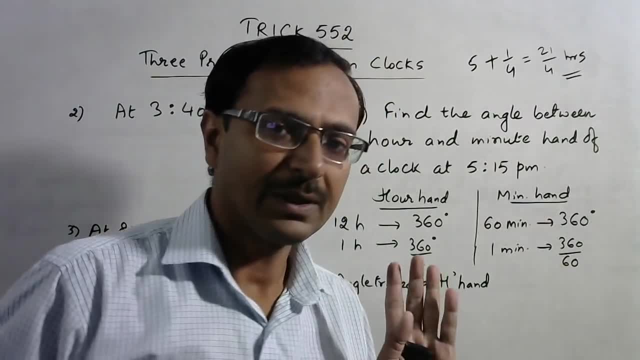 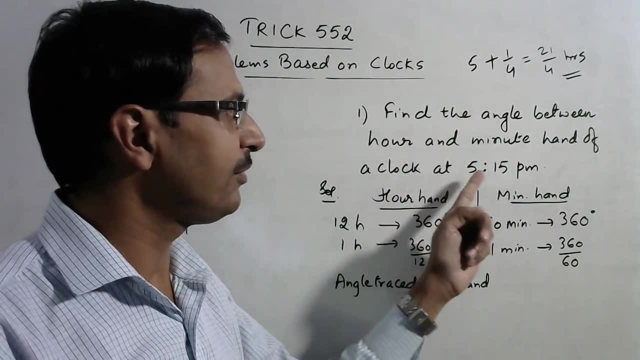 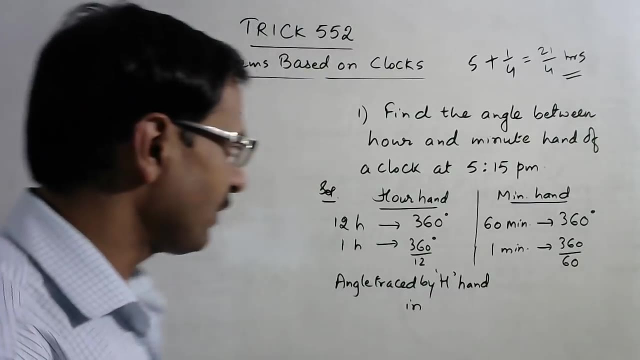 by 4 hours. So actually the hour hand travels from 12 and covers 5 full hours plus a quarter hour. That is 21 by 4 hours. So we will find the angle traced by r hand in 21 by 4 r's. 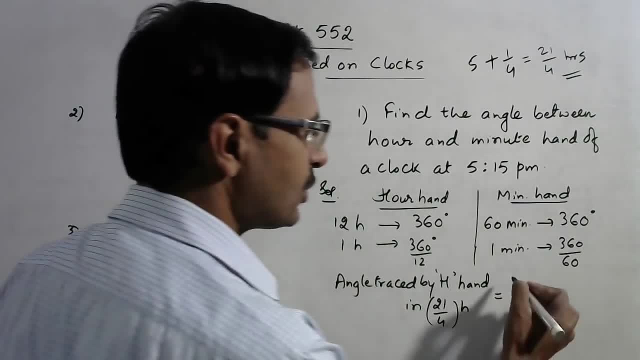 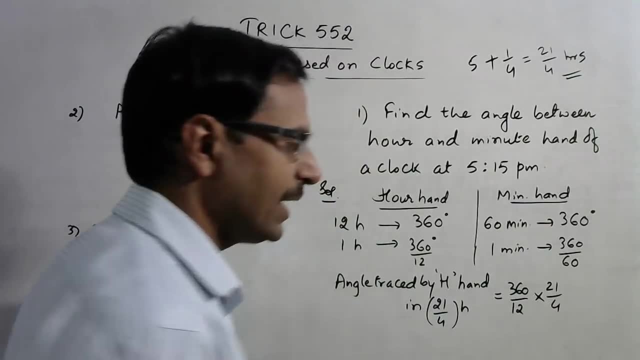 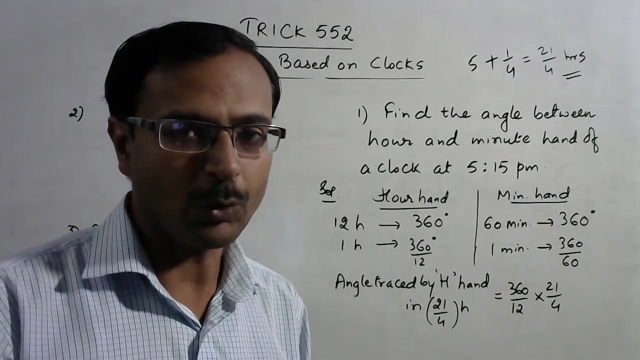 Now, what is the angle traced in 1 r? It is 360 upon 12.. So simply multiply this quantity by 360, by 12 and you get the angle traced by the r hand. A very simple concept, and you need to understand this concept if you want to solve the problems comfortably. 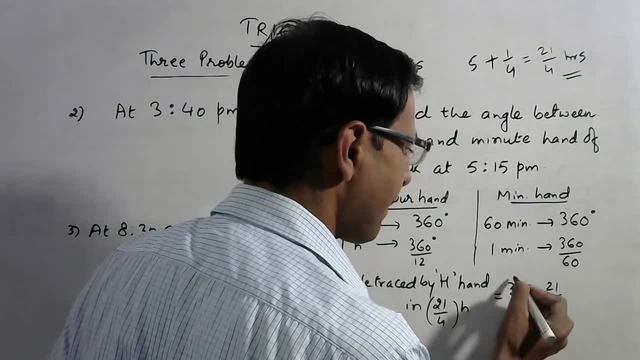 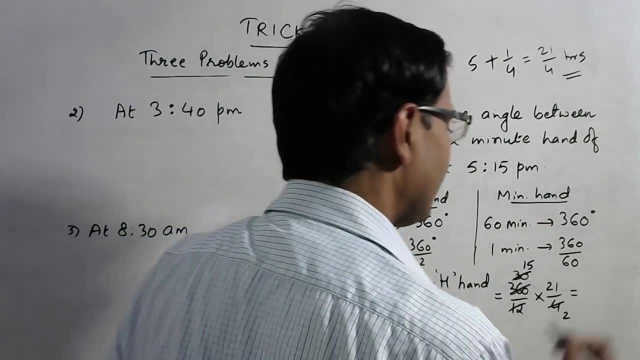 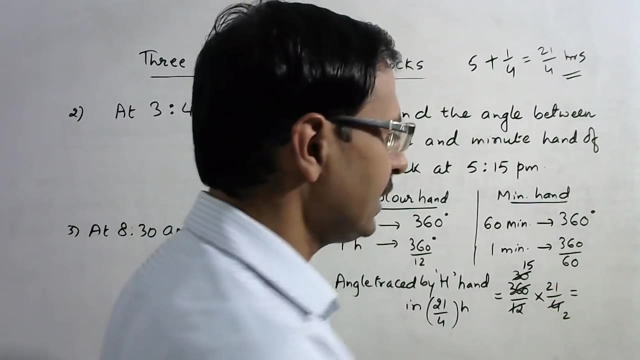 See, this is 30 and you can still divide by 2.. So 15 into 21.. 15 into 20 is 300 plus 15, 315 by 2.. So this is 157.5 degree. 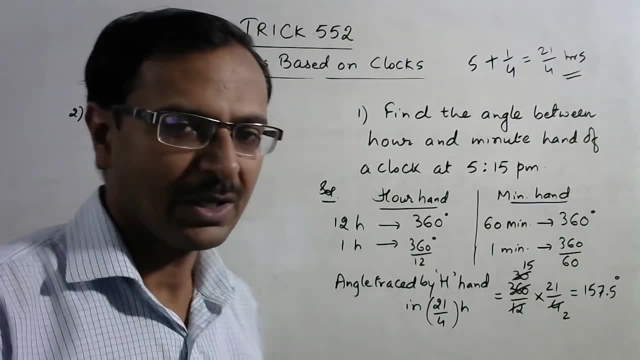 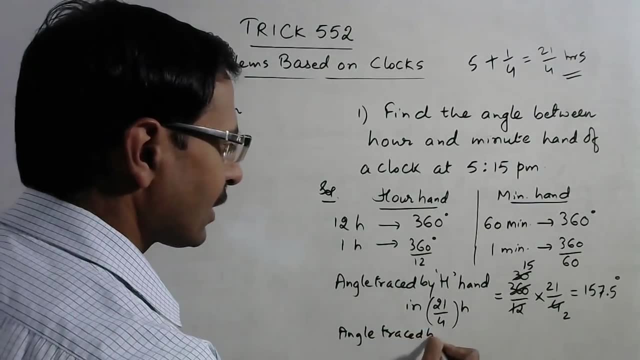 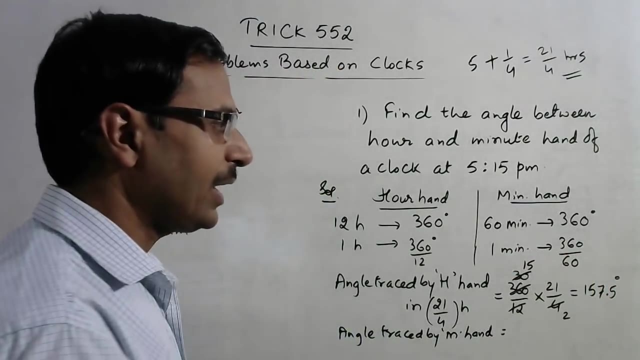 Now, that is the angle traced by the r hand. Now come to the minute hand. So, angle traced by minute hand. Now, what to do In 1 minute? it is this much, Now, in how many minutes we want to find. 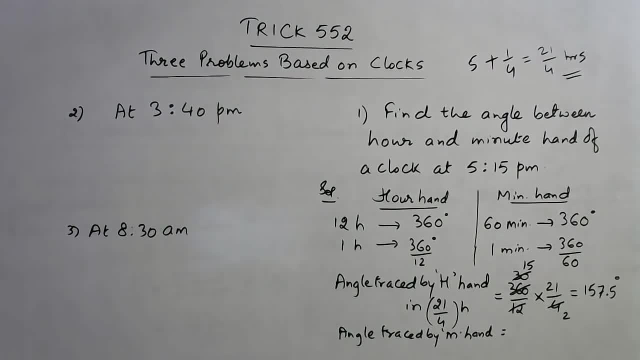 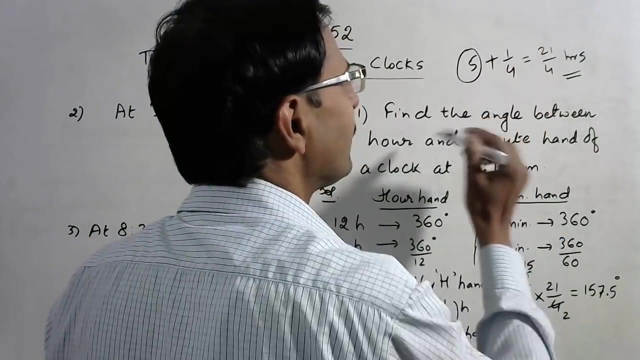 That is a question of importance here. Now see, the time which we have taken is 21, by 4 hours in case of r hand, But in case of minute hand, just forget this. This is complete hours. We have only 15 minutes. 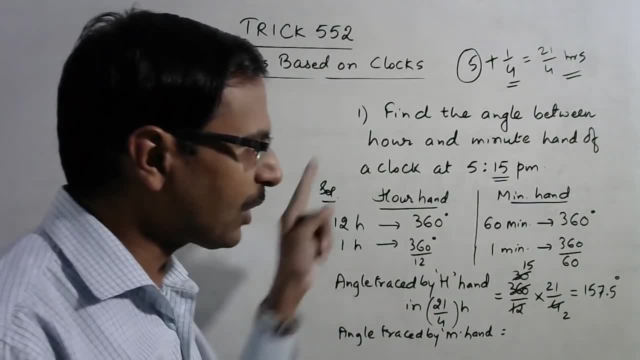 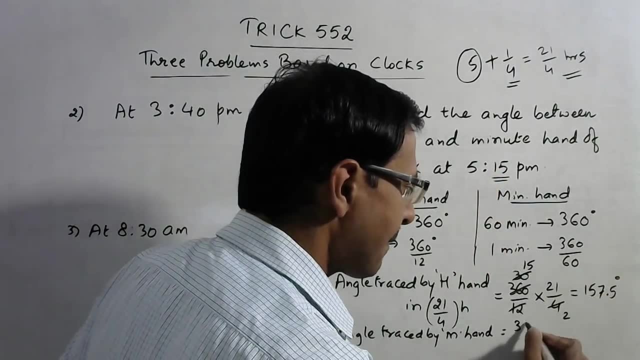 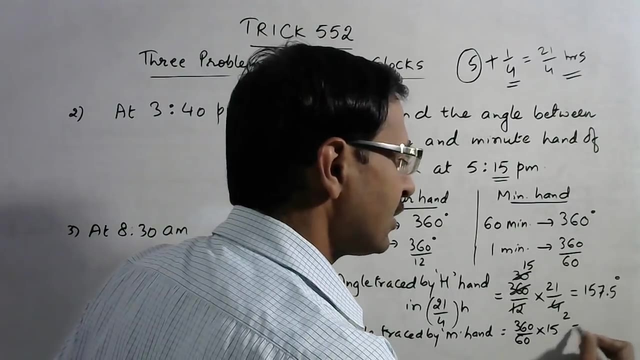 So actually 5 complete rounds for 5 hours and for 15 minutes. we need to find the angle traced, So 360 by 60.. That is already there. Just multiply it by the complete minutes given in the question, So that is 15.. 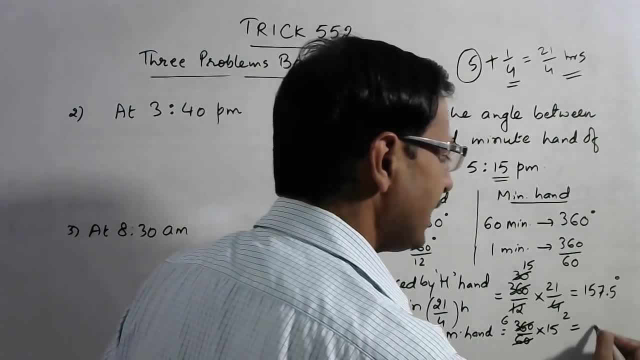 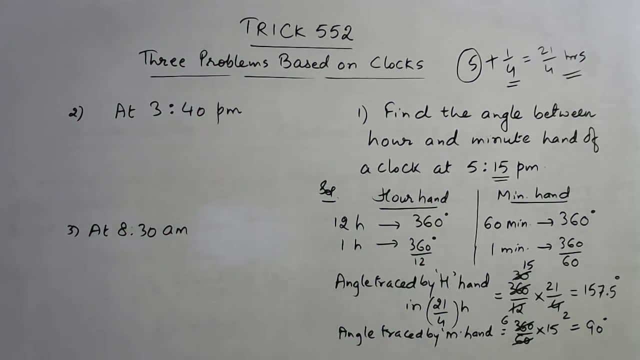 So now you can find this. This is exactly 6.. So 90 degree. Now we have the angle traced by the r hand As 157.5 degrees, And the angle traced by the minute hand is 90 degree. 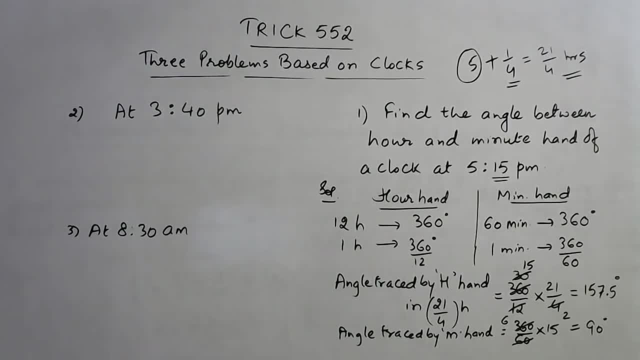 Now to find the difference, just subtract the two angles. We will get the answer for our question. So required angle is the difference of 157.5 and 90,, which comes out to be 67.5 degree. This is the answer for our question. 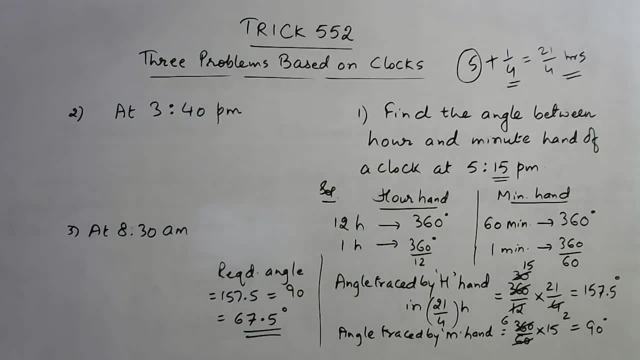 Okay, answer for our question. Now let us take one more time. This is 3.40 pm. For 3.40 pm again, we will use the same concept, So angle traced by the R hand in. Now that is important. How much time it is given Now, see 3.40. 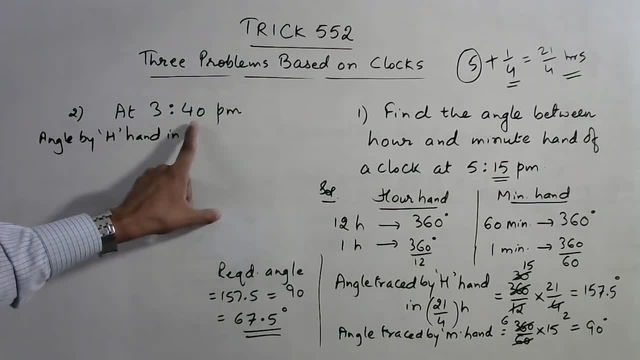 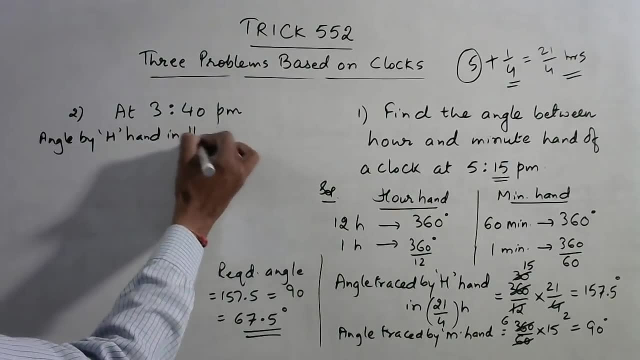 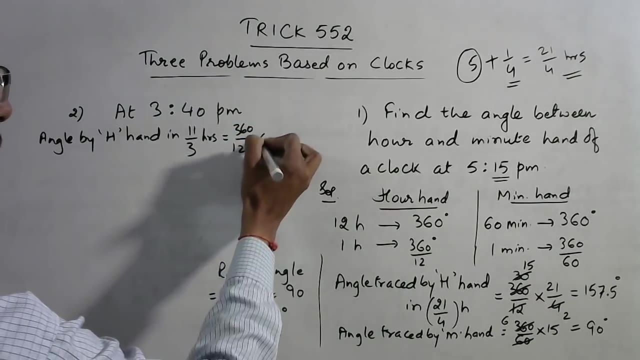 means 3 complete hours plus 2 by 3 hours. 40 minutes is 2 by 3 hours. So 3 plus 2 by 3 is 11 by 3 hours. Now what do we do? We just multiply this by 360 by 12.. So this goes exactly. 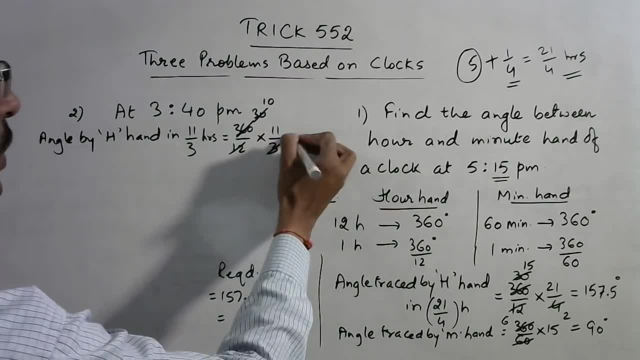 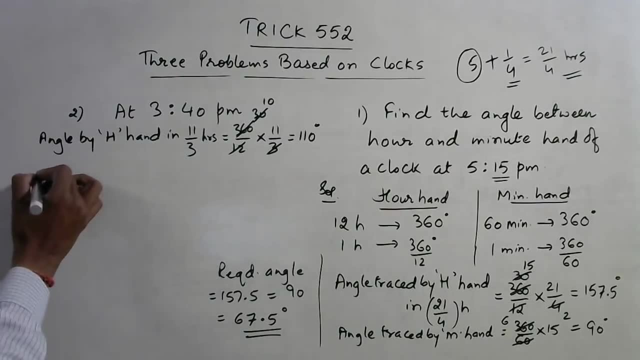 30 times. This goes 10 times. So 100 and 10 degree is the angle covered by the R hand at 3.40 pm. Now the angle covered by minute hand. Now I told you for minute hand we do not consider the. 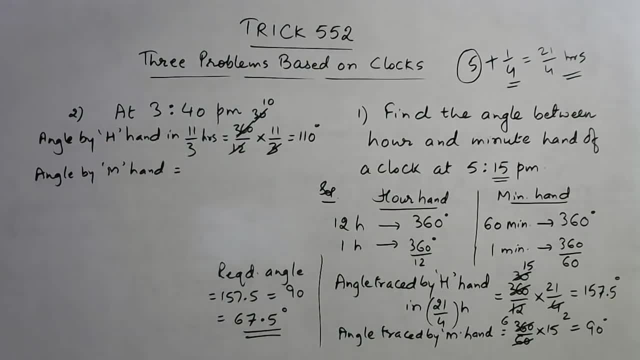 complete hours. We just see the minutes. The minutes given here are 40. So multiply that by 360 upon 60. You will get the answer. for minutes, This is 240 degree. Now the question is very simple Once we get. 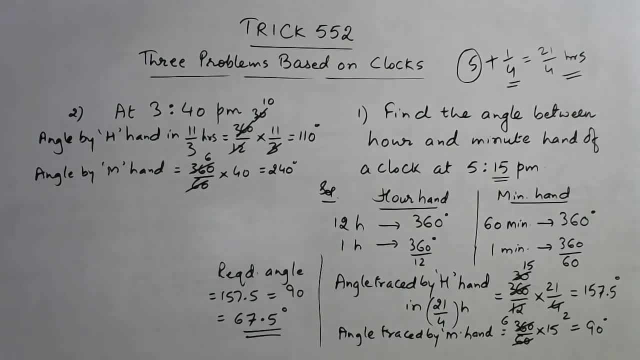 both the angles correct, then only thing is to find the difference between the angles. So the required angle will be difference between these two. That is 240 degree minus 110 degree, That is 130 degree. is the answer. Now you can take more questions like this. Suppose: 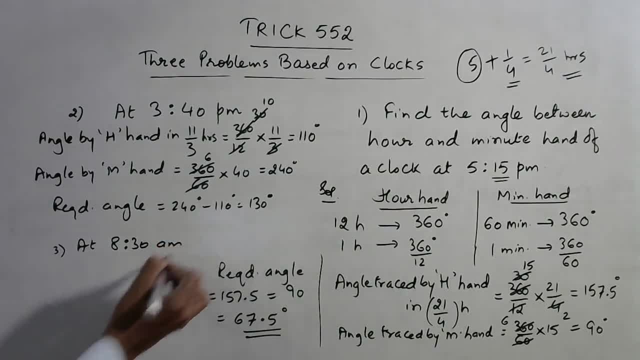 you want to find at 8.30 am, Again at 8.30 am. use the same concept. I am sure you will be able to solve this question yourself now. Now 8 and half. So for R hand. 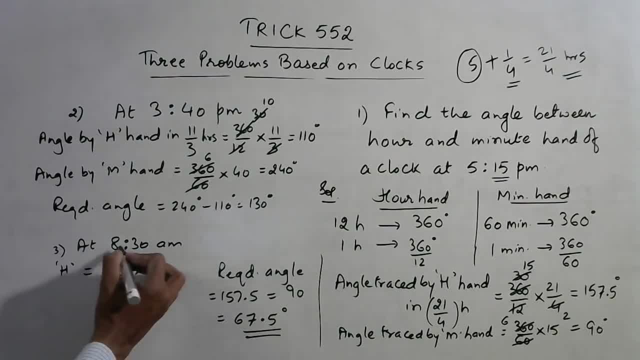 the angle will be 360 upon 12 multiplied by 8 and half. 8 and half means 17 by 2.. Now you can cancel this. If you solve this, this will come out to be 255 degree, And similarly for minute hand. 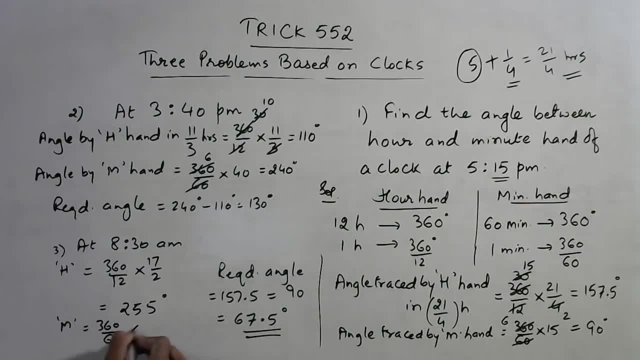 360 upon 60, multiplied by complete minutes. 30 minutes is 30 here, So this goes 6 times. So 180 degree. Now just find the required angle. Required angle will be the difference between these two, So the answer will be: 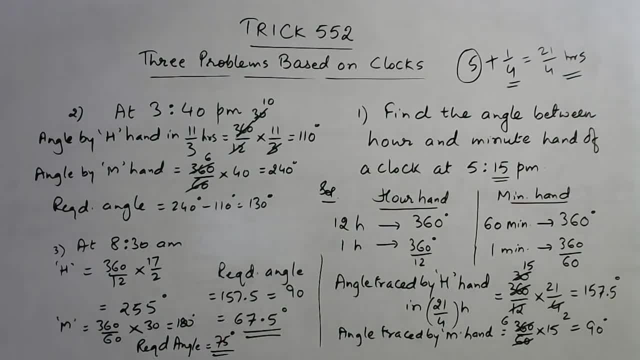 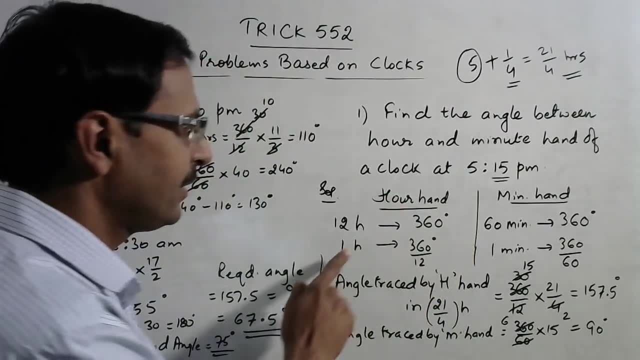 75 degree. Likewise, you can go on and on. Take any time of your choice. Use this concept that in case of R hand in 1 hour, the angle covered is 30 degree And for minute hand, the angle covered is 1 minute. So you can go on and on. So you can go on and on. So 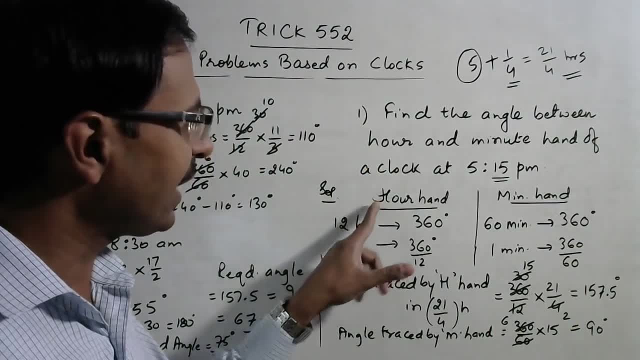 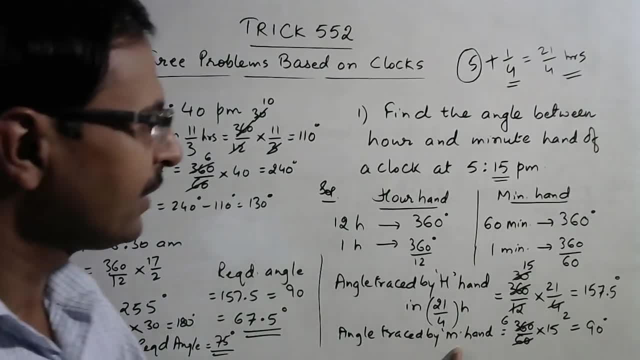 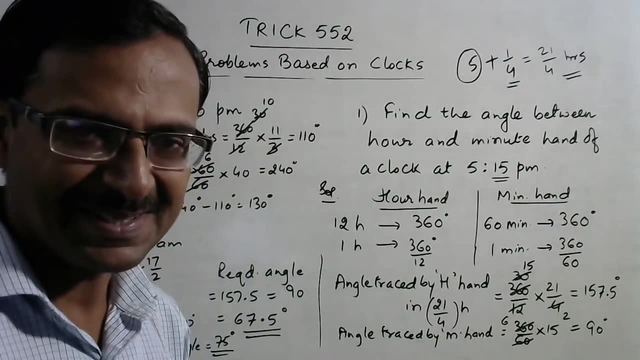 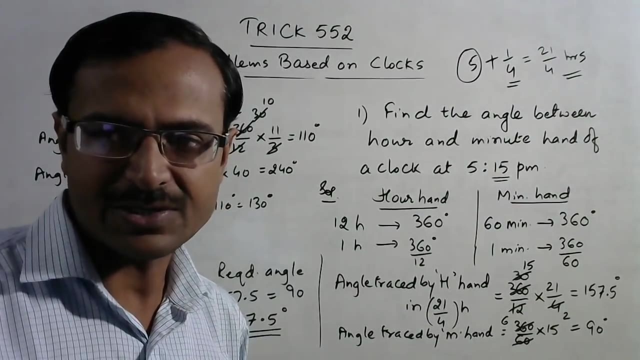 here And in case of the minute hand, just take the complete minutes. Forget the hours. Just take the complete minutes and multiply that by 360 upon 60. So this is a very important concept for NTSC exams. Also, banking, RR, BCGL, SSE, all exams you find such questions.